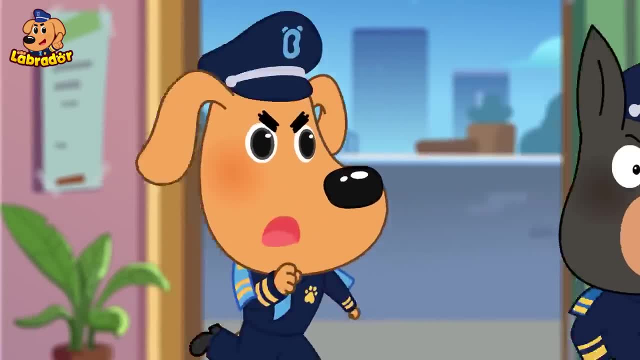 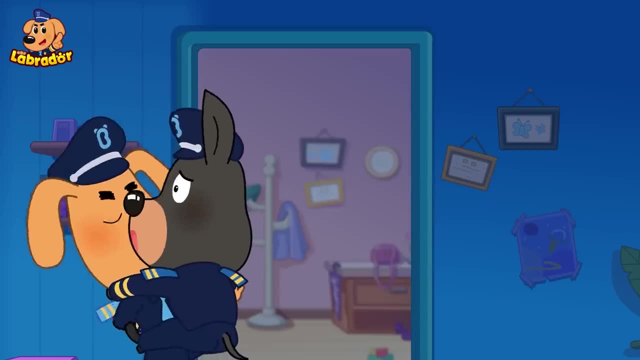 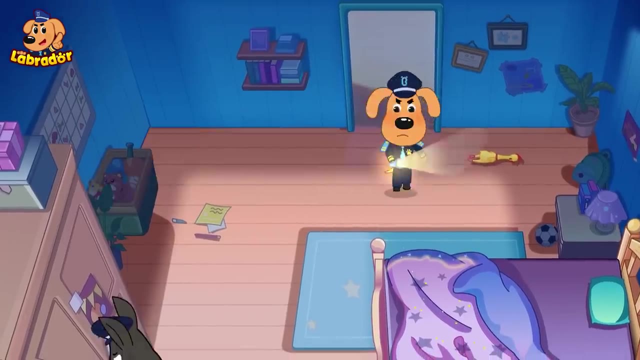 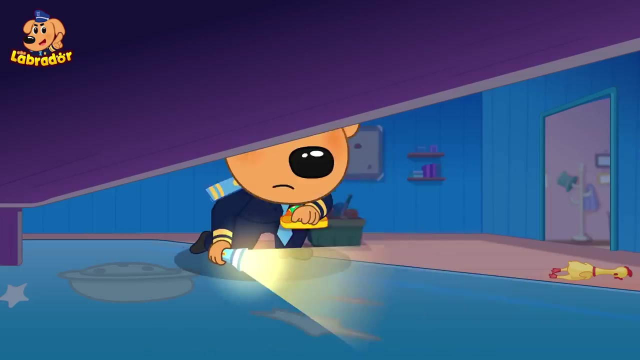 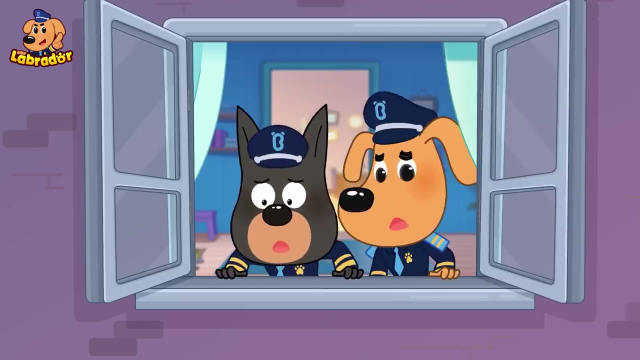 Don't worry, there's no case that I can't solve. Dobie, you stepped on a toy. Oops, This is Little Gekko's slipper, But where's the other one? It's a ghost Run, Ouch. 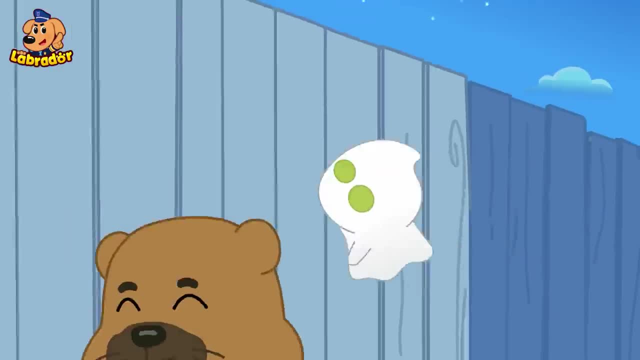 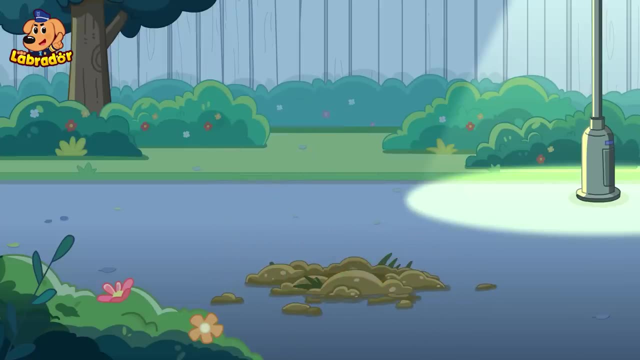 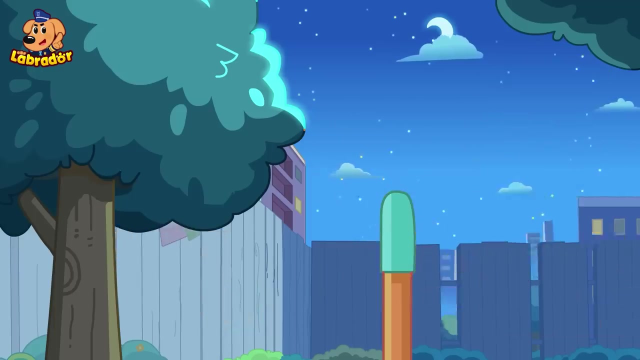 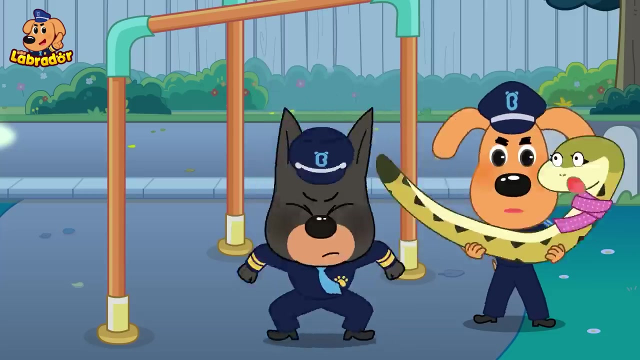 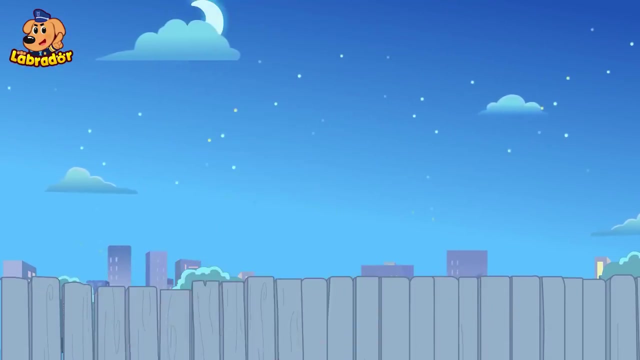 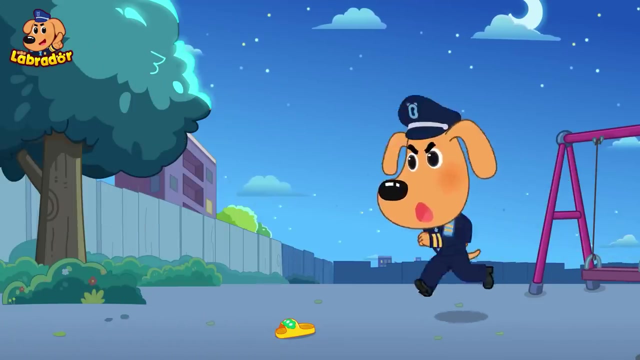 There is a ghost, Let's go have a look. Ah, Ghost, Oh, it's a ghost. A ghost It's over there, Who's pretending to be a ghost And even hitting me with a slipper. This is Little Gekko's slipper. 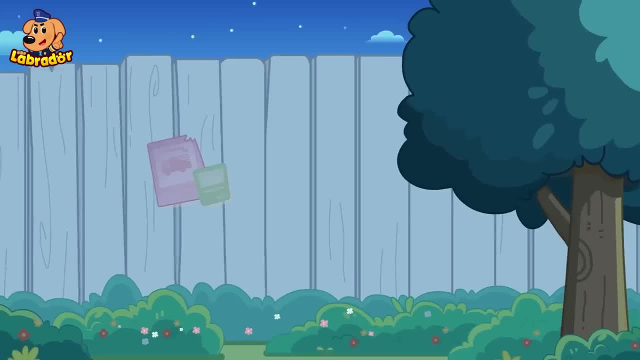 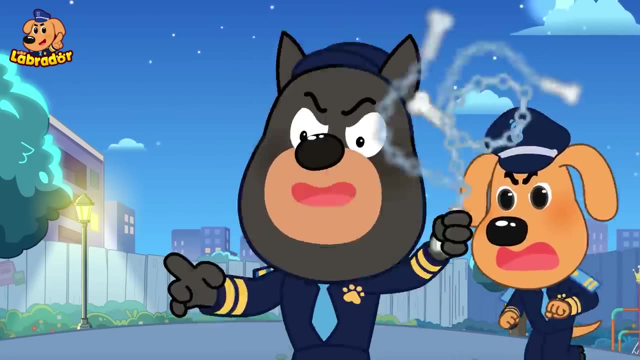 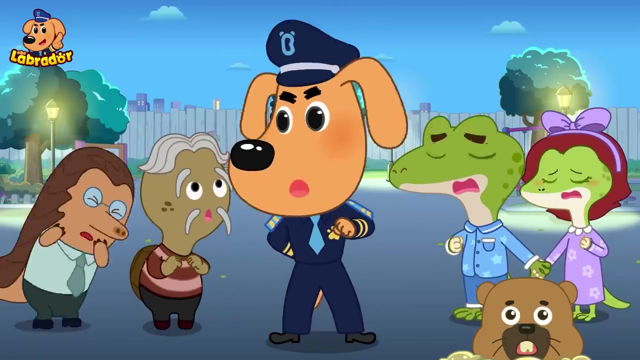 Let's go find out. You can't run away, Dobie, stop. Why did you let it get away? That's not a ghost, it's Little Gekko. That's not a ghost, it's Little Gekko. 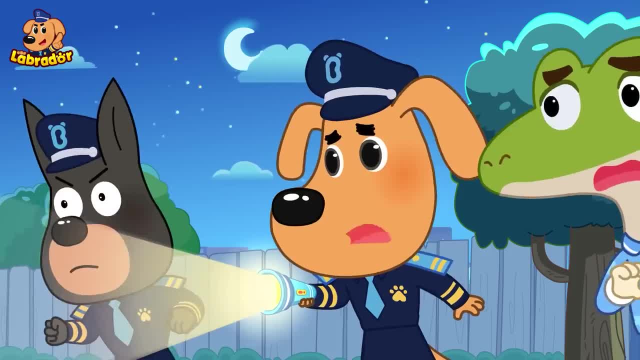 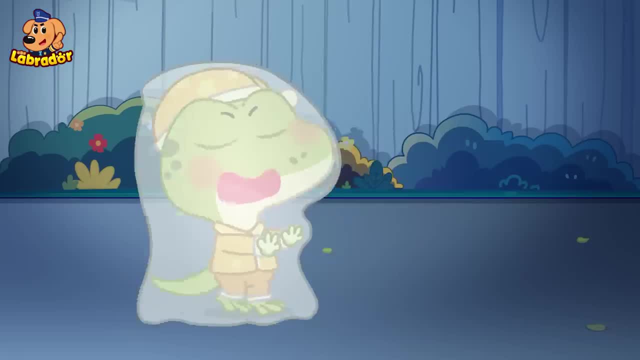 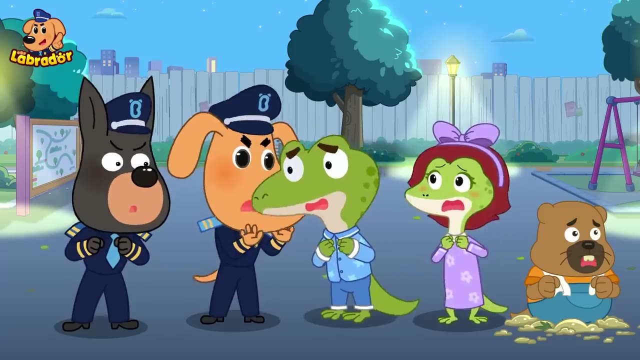 What's going on with him? Looks like he's sleepwalking, Sleepwalking. Then I'll go wake him up. No, It could be dangerous to wake him up now. Ah, He's climbing up the wall, My son, Don't worry, we'll take him home safely.